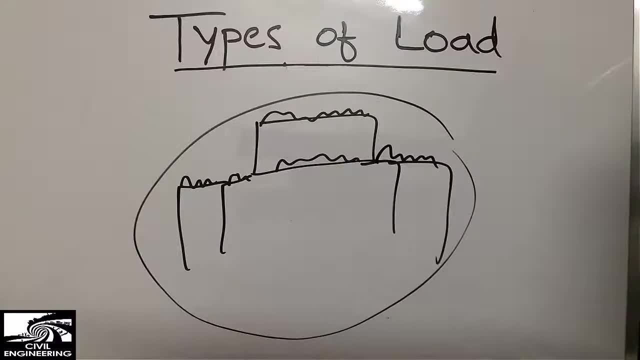 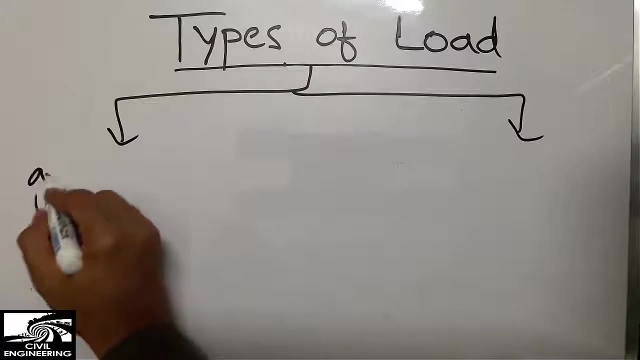 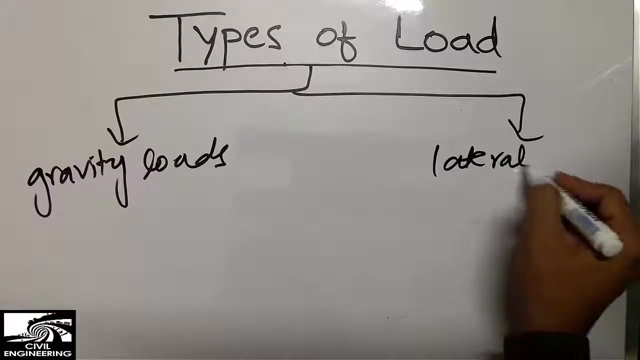 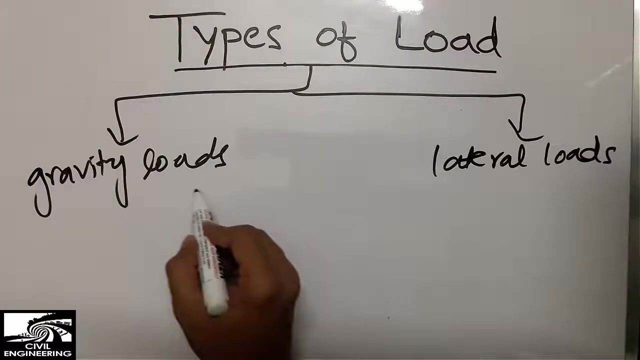 So we are going here to classify what are these types of loads. There are mainly two types of loads acting on the structure. One is the gravity loads and the other is lateral loads. Right, so what are the gravity loads? Gravity loads are those loads like I am drawing here. it is a beam and let's suppose it is a car. 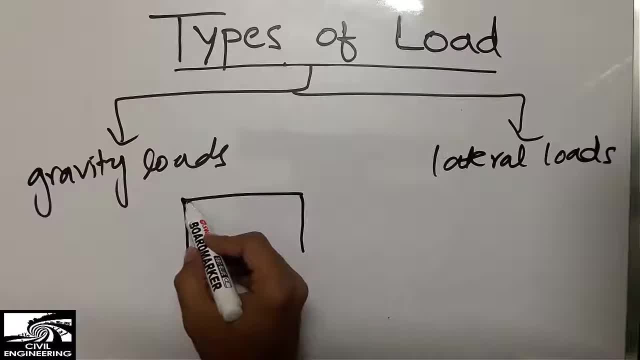 Let's suppose it is a column and it is a frame structure, So the loads that are acting in the downward direction, in the direction of gravity. its name shows that these loads are acting in the gravity direction, So we call it the gravity loads. 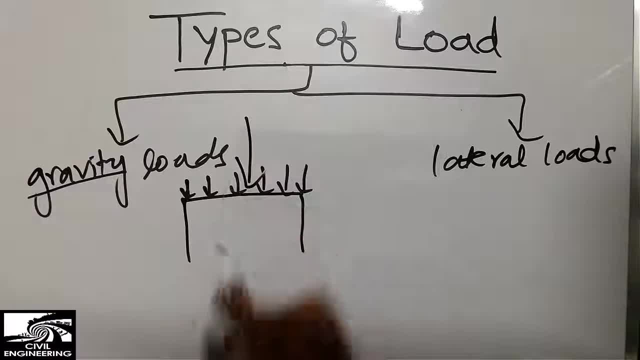 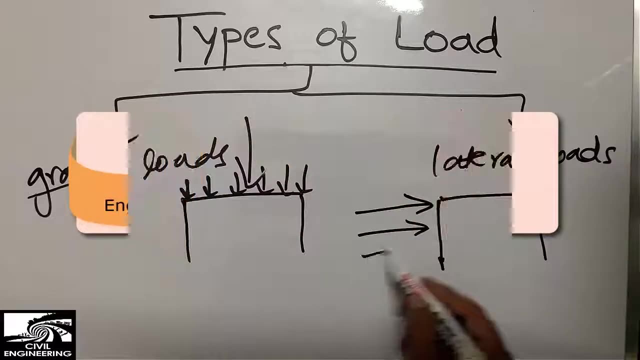 Right, those loads which are acting in the downward direction we call as gravity loads, While the lateral load is totally different from that of the gravity loads. these are the loads. I am taking an example of the frame structure. The lateral loads are the loads that are acting on the structure and in the lateral direction, in the horizontal direction, we can say: 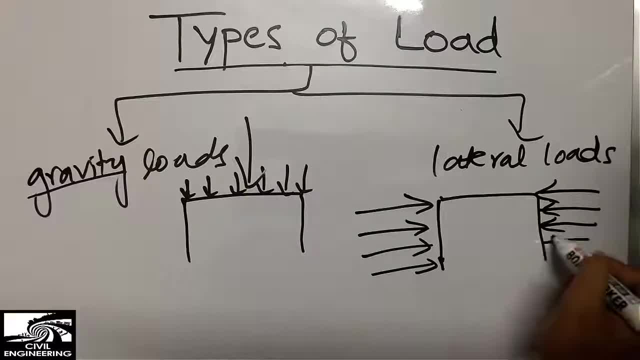 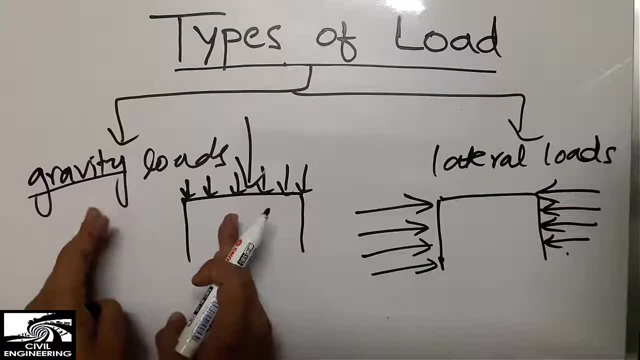 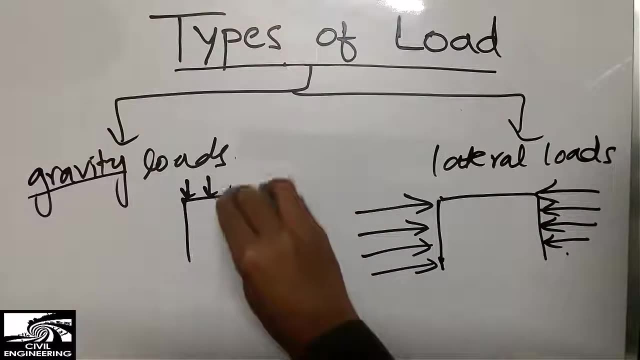 Right. so these are the type. these loads are included in the lateral loads. Right. so one is the vertical loads- gravity loads- and one is the horizontal loads- we call it lateral loads. Right. so now again classifying the gravity as well as the lateral loads in a further classification in these two types of loads. 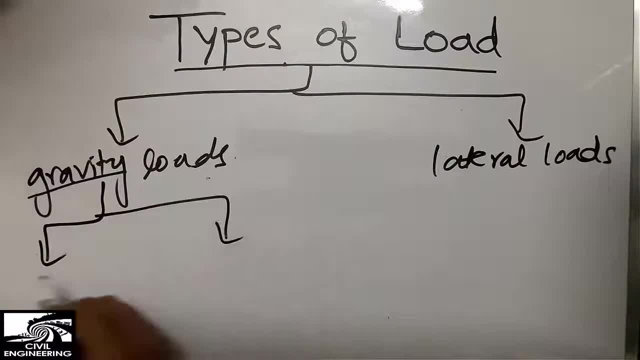 And the gravity loads. we have two other classifications. One is the dead load and one is live load. Right and the dead load we have like the load of the furniture. we can say These are the loads which do not change with time or with position. 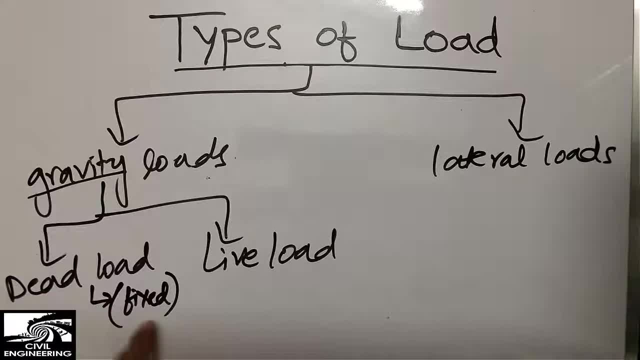 It is fixed on a member. We call it dead load. This may be the load, The surface of the structure. we call it the dead load because it is not changing, going to change. And dead load may include the furniture load because the furniture is fixed on the structure throughout the year. 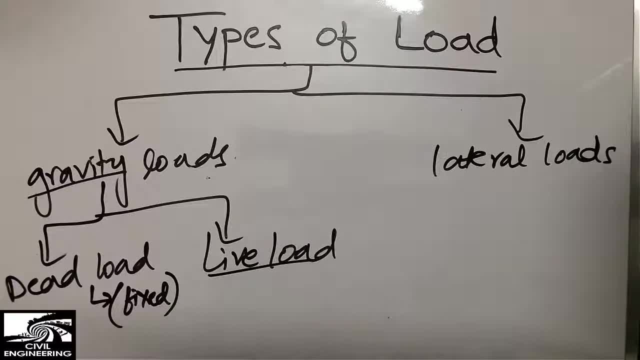 So we call it dead load, While the live load, the live loads are those which are going to change in position, So we can say change which are going to change in its position, like the people moving on the floor. on the second floor.